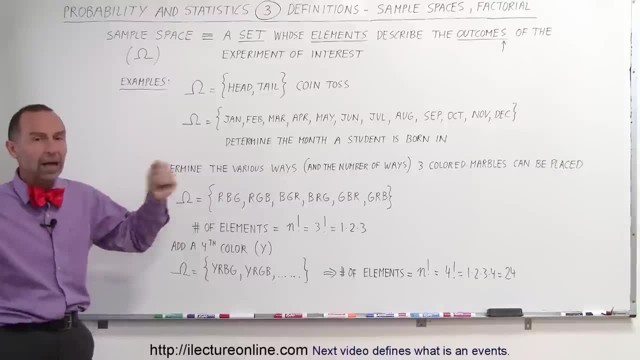 no other than the twelve months there, so that encompasses all the possible outcomes. so therefore, this is the sample space, the set of all the possible outcomes of the experiment. the test determining what month a student is born in Now determine the various ways. 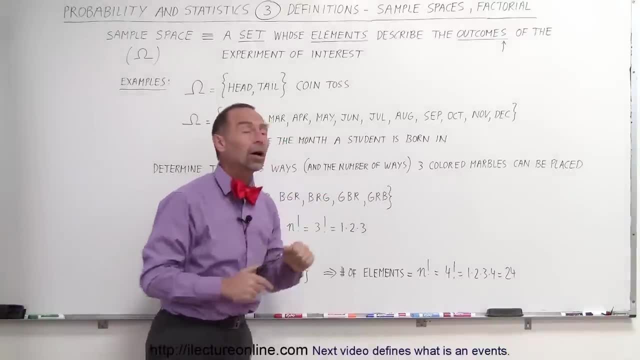 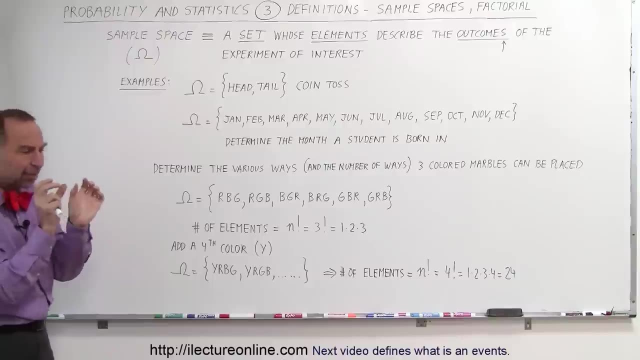 that we can line up three colored marbles. Now that's a different kind of sample space. so what are all the possible ways in which we can take three different colored marbles and line them up in a certain order? Well, let's say we have a red one, a blue one and 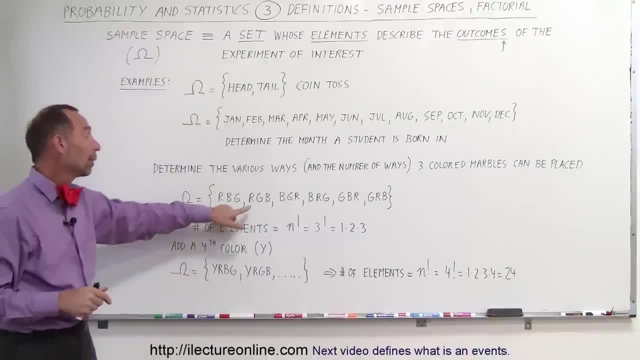 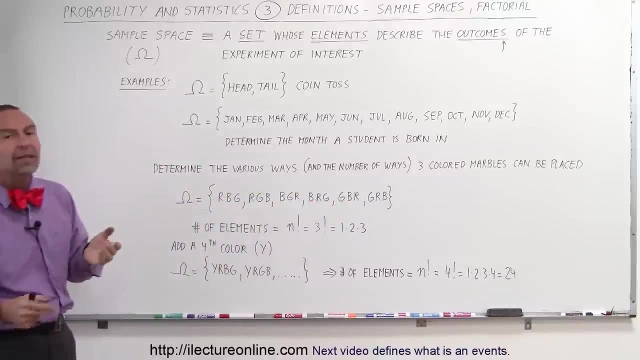 a green one, so we can have red first, then blue, then green, or red first, then green, then blue, or the blue first, then green, red and so forth. And notice there are six different possibilities in which way we can line up those three colored marbles. So let's. 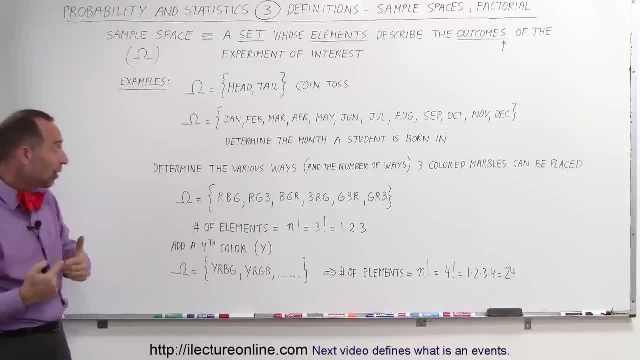 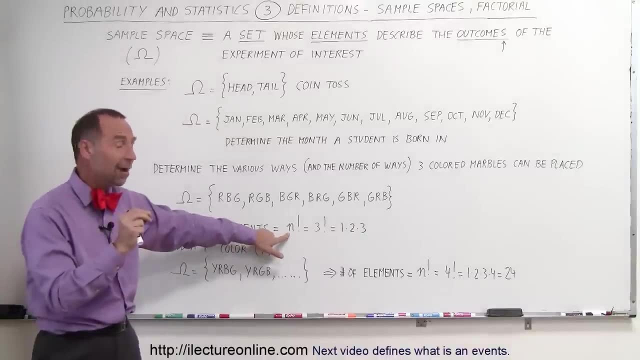 say, we have three colored marbles. The way we can find out how many possibilities there are, we can simply say: the number of elements, the number of outcomes or possibilities is equal to the number of marbles that we have, in this case three factorial. Now what does? 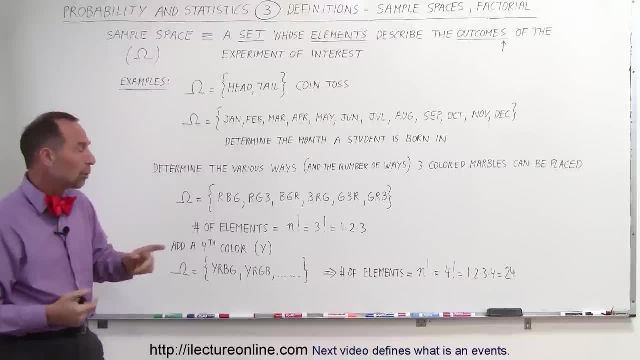 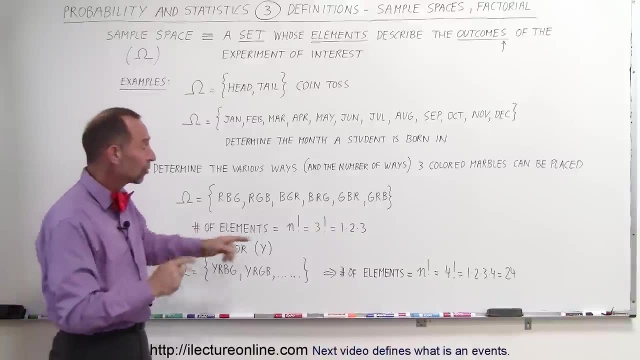 that mean factorial. Well, if there's three factorial, then we multiply the number one times the number, two times the number three. Sometimes they start with number three and work their way down. doesn't really matter, as long as you multiply them together. So 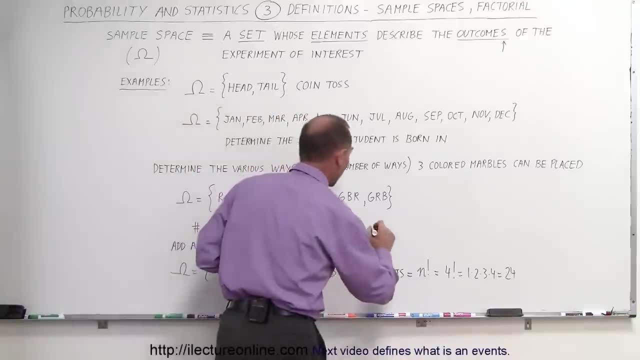 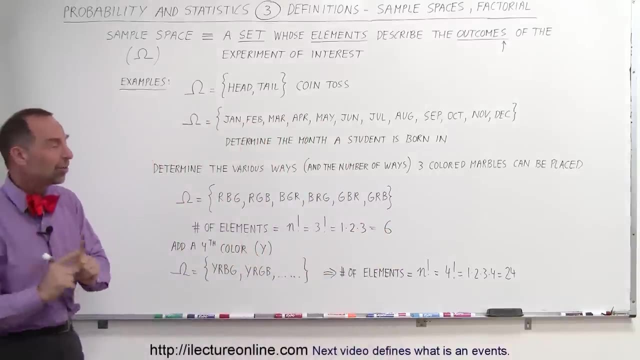 three. factorial is one times two times three. when you add all that up or when you add more, When you multiply all that together, you get six. So therefore there are six possible outcomes. therefore, there are six elements in this particular sample space. What if you add another marble? 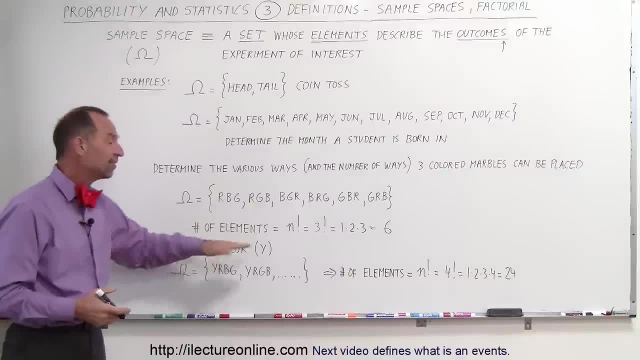 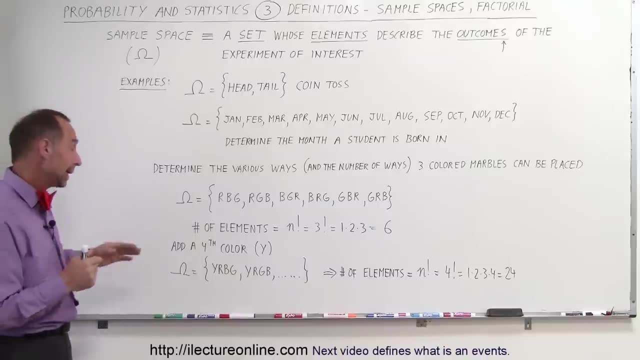 Now you have four of them. Let's say, the fourth marble is now yellow. So now we have a yellow, a blue, a green and a red marble. How many different ways can we line them up? And again, you can start out by putting the yellow first, then the red, then the blue, then the green. 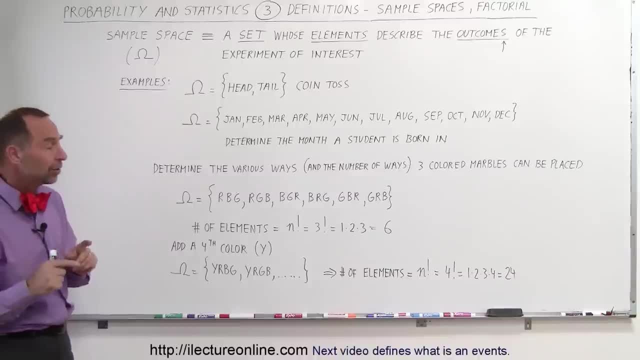 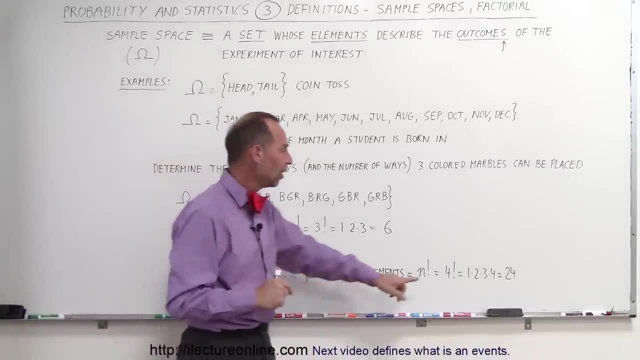 then the yellow, red, green, blue and so forth. How many possibilities are there? Well, in that case there's four marbles. So you say four factorial is the total number of outcomes, the total number of elements. Four factorial is one times two times, three times. 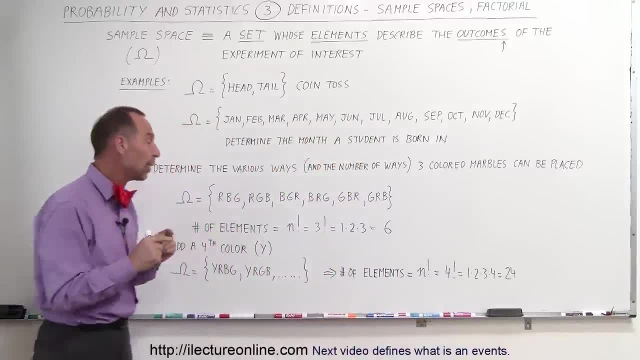 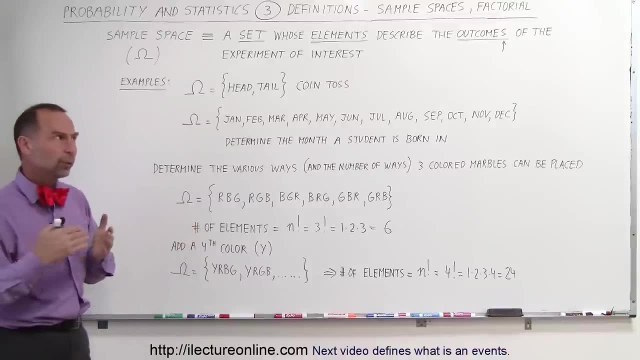 four, which is equal to 24.. So there are 24 different ways in which you can line up four different color marbles. What about five different color marbles? That would be five factorial. Ooh, that would be 120 different ways. So that's how we determine that and that's what.